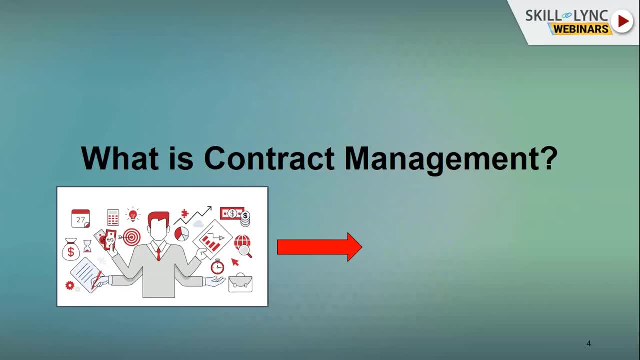 so definitely that project will be ended in a good terms for particular owner or a customer, or for the contractor also. But there are certain cases. there are certain cases where you know the project was not handled carefully. then it is a firefighting for both the parties. 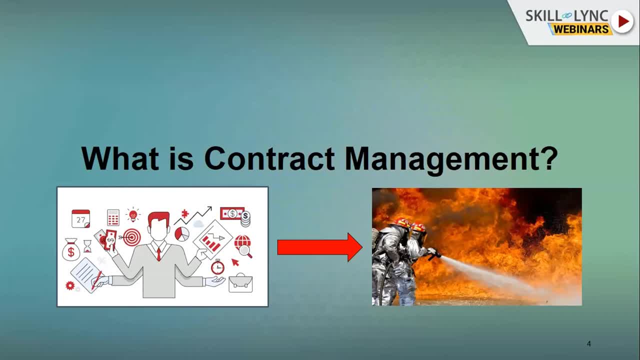 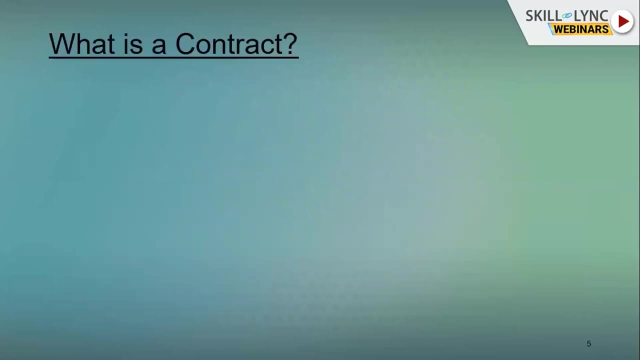 Example for owner as well as for the contract. So the second image is shown that you know that if you will not handle the project start to end in a proper manner or with the proper skillset, it will. it is disaster for everyone. So, to start with, can anyone tell me about what is the meaning of a contract? 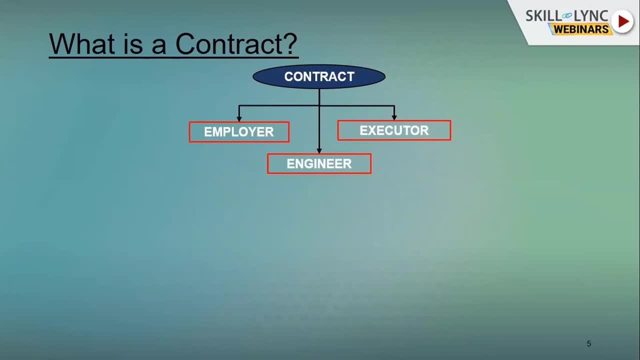 Okay, No problem. So I will say that you know that you must be having doubt that you know the this contract management. it is very difficult to handle, or do we need to spend some time and money for it? So the answer would be definitely yes, because proper skillset and knowledge and experience. 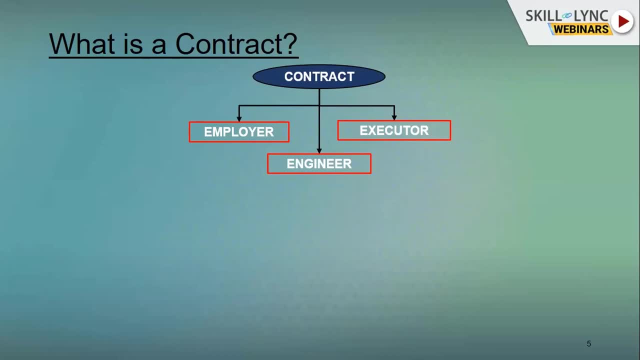 is much for the contract manager, And this is continuously growing process, or a continuous improvement process, where experience also plays a major role. So what is the contract? Contract is nothing but a return, or a return or a oral agreement between employer, engineer and executor. 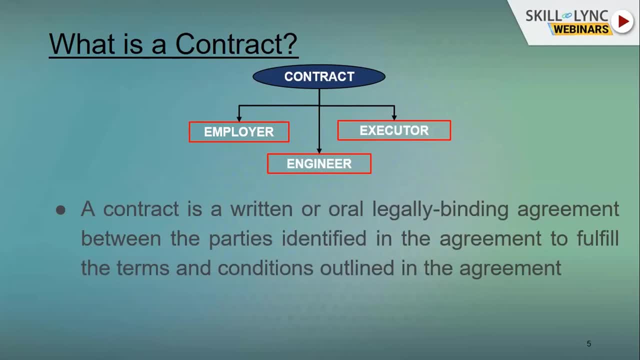 So your employer is nothing but the owner, or a customer Executor is nothing but the contractor and engineer is. in our terms, in civil engineering construction term, It will be called as a PMC. Yeah, There are chances Where the employer is competent enough to not to not to have with the PMC in the contract. 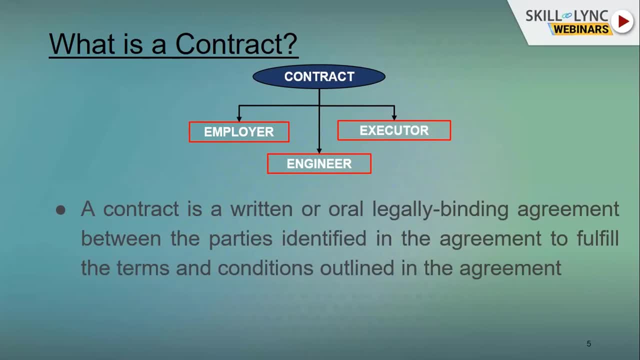 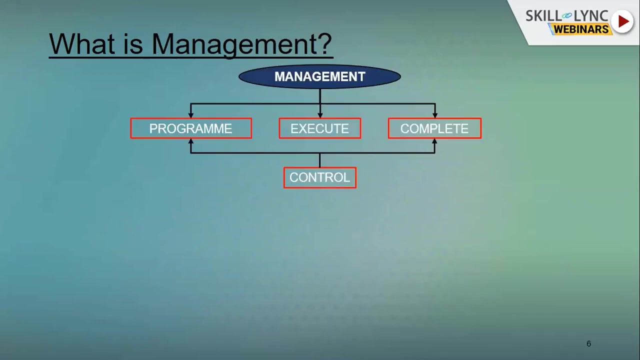 So they will directly do the contract to the executor, where PMC will not be tasked. But this is a general, typical funda, where the majority of project are having all those three party in a contract. Yeah, So, as you know, everyone knows that management is nothing but two. 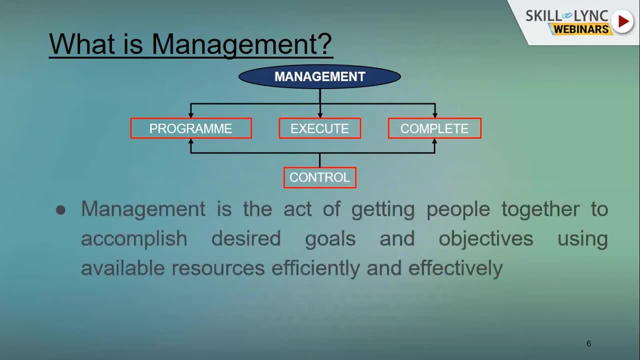 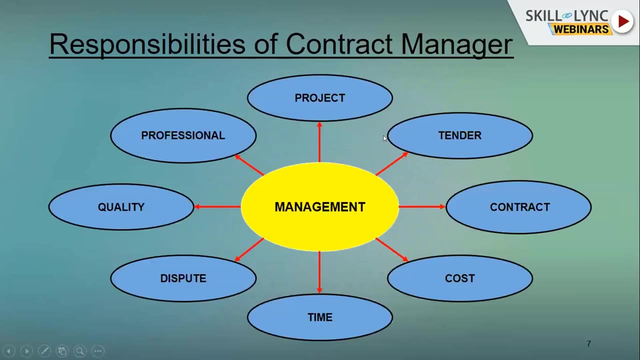 Yeah, So it's not like you have to plan something, to execute something and to complete something which is as per the owner or a customer demand. So, definitely, management is the act of getting people together to accomplish desired goal, as everyone knows that. So so now to proceed further. actually, I would like to show you that. what are the responsibilities? 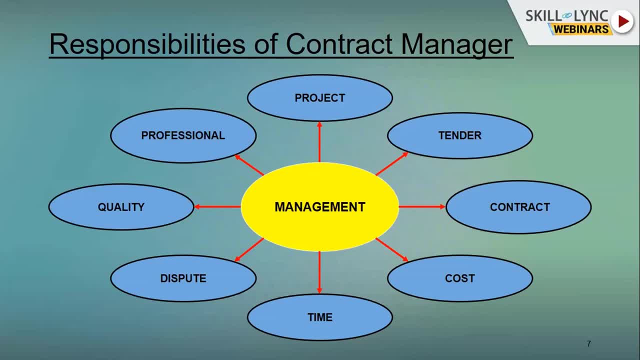 of a contractor manager. So the start with you know any owner or any owner. So the start with you know any owner or any owner. So the start with you know any owner or any owner. Okay, So uh see, you offer company will tell you being a contract manager of the company. they 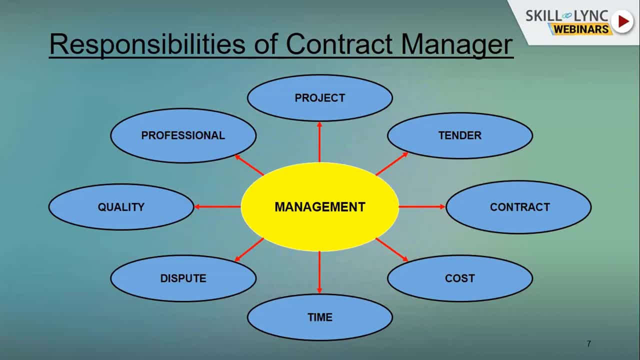 will give you the project name, details and everything. The walk starts with the tender, followed by the contract, allocation of the time, etcetera, etcetera. We have to handle or the carry out the project within desire, quality, And definitely no one will going to go into dispute because dispute is a major or a vast 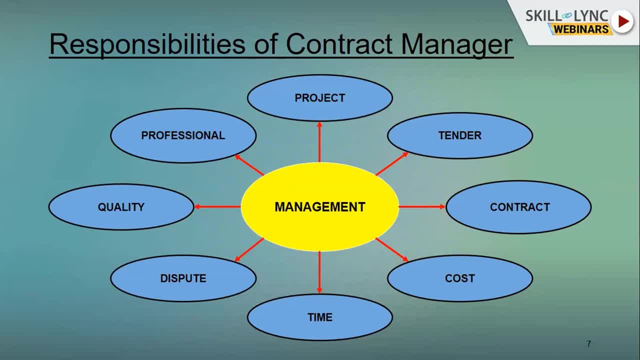 topic management, we can say that no one, either of the party, wants to go into that particular field because commercially, financially as well as you know your name and fame, everything will be on a sake when you are going for the dispute. but that is also a major part where contract manager has 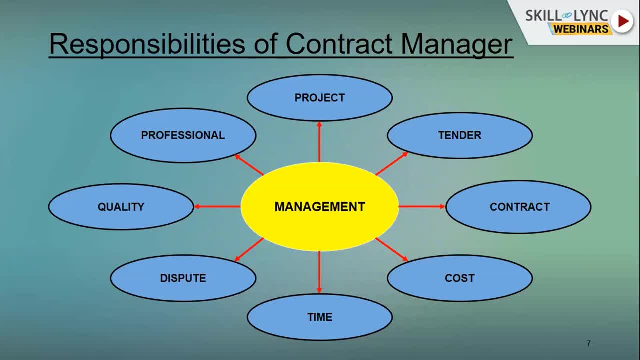 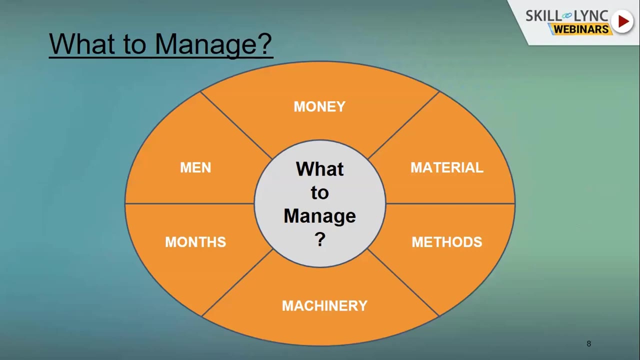 to think that you know to, in the benefit of the owner or a CEO or a company, that if it is going, then how the dispute management has to be handled from their side. so to proceed, that what, what, what is to be managed at the site level for a contract manager? so he has to manage definitely six aim. 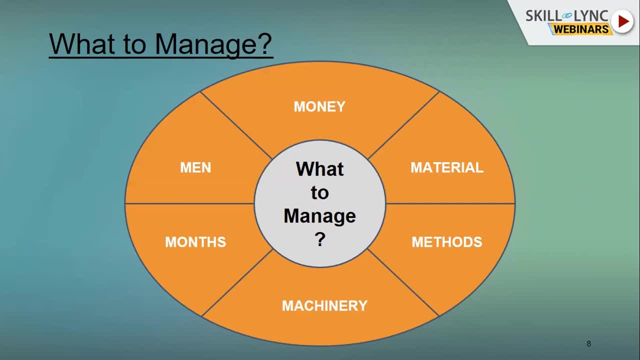 related to construction industry: money, material, methodology, machinery and months and men. so this is all we know. but you know, the management of all this entire, from beginning of the project to mid of the project, to end of the project and to till handing over it- is very difficult every. 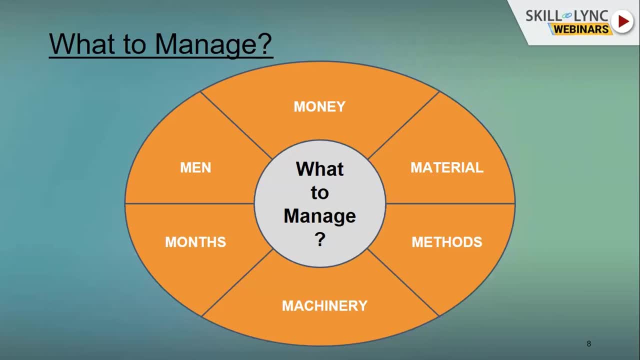 aspect has its own skill set to handle on knowledgeable person. or sometimes do happen that you know that the contract manager must not, maybe not having the correct idea about the methodology. so there are team members inside in the team that they will guide you, they will do the work for you, they will give you the better ideas so that 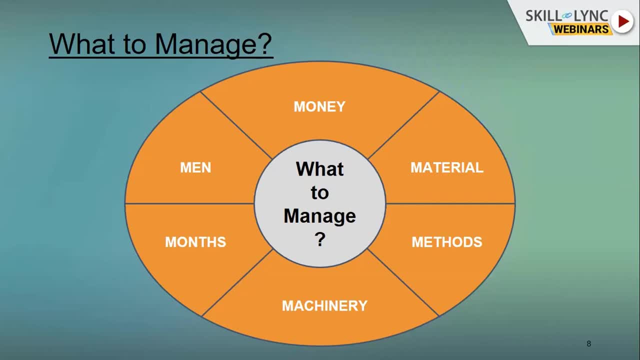 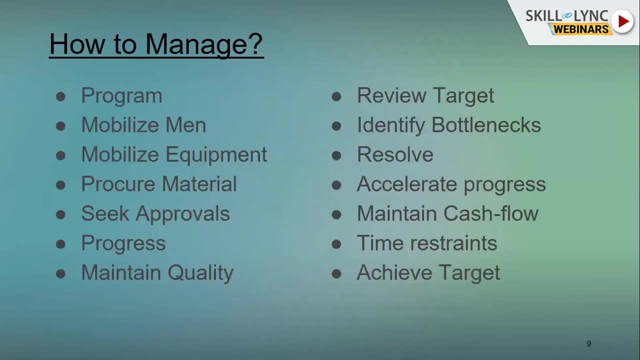 contract manager has to be very open for the different ideas and he has to accept it to achieve the desired goal set by the company. I have mentioned that once you know you will be asked to come out, you will be asked for a certain project, so how you will going to go. so we will take a. 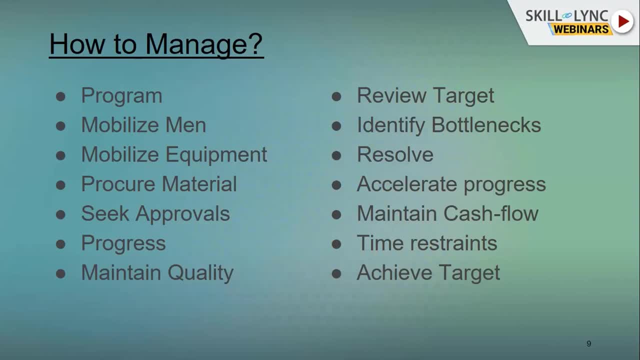 foundation of a G plus 40 building tower as your project and we will start as a one step of foundation. so, say example, we will going to plan the foundation that starting from the scenario that whether that property is clear to start the work, whether that property is having 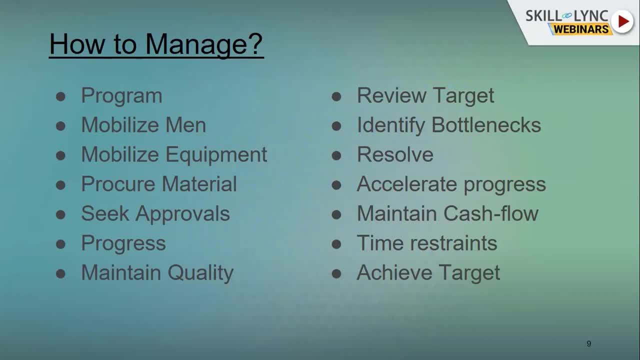 any, any government issue. do we have the CC to start the work? do we have the proper manpower, do we have the proper machineries, etc. etc. accordingly, he will going to make a program and accordingly, he will going to manage the different materials to get at the site and to and. 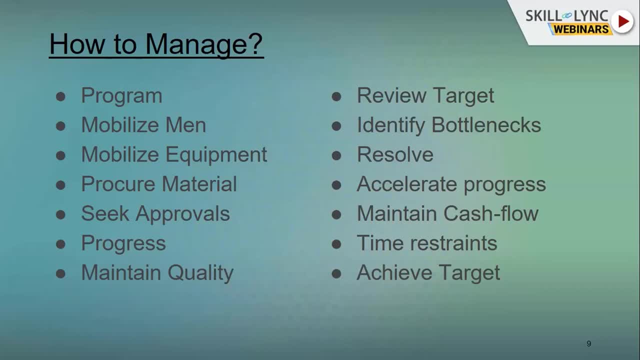 to give a proper progress. but in the mean time definitely he has to target some bottlenecks. say example, if we are doing a foundation work in the moon soon, the major bottlenecks is nothing but the water logging in the whole in the excavated area because, uh, that are the major bottlenecks. so try. 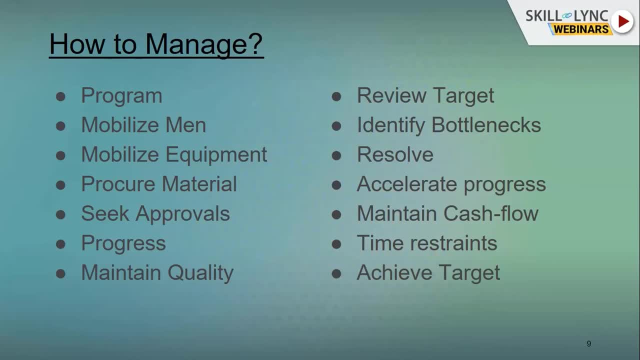 to plan in that way that you know majorly your work of the foundation is not going to have a lot of can be completed before the monsoon or you will start after the monsoon. so such a planning gives you the experience as well as the knowledge what kind of works. 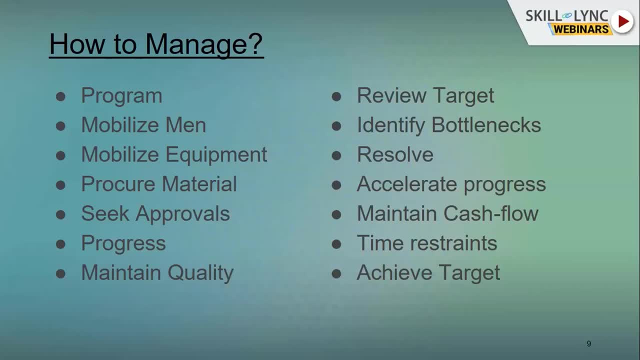 that you will going to target in which season that everything should be plan in the initial stage, better way to identify the bottlenecks and accordingly we will resolve the issues. and the second most important point, that you know that how will going to accelerate or how will going to recover the delay because, say, 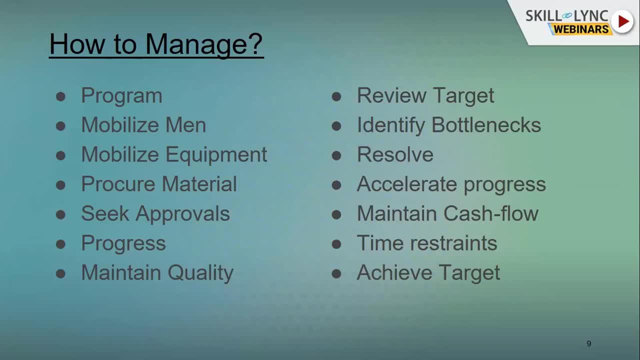 example pandemic. no one has come. you know, consider this pandemic has last for almost one and half years till now and I don't know how it will go further. so such an unexpected, unexpected, a planner, unexpected things will come and target your competencies. so how that particular things will going to come and affect our 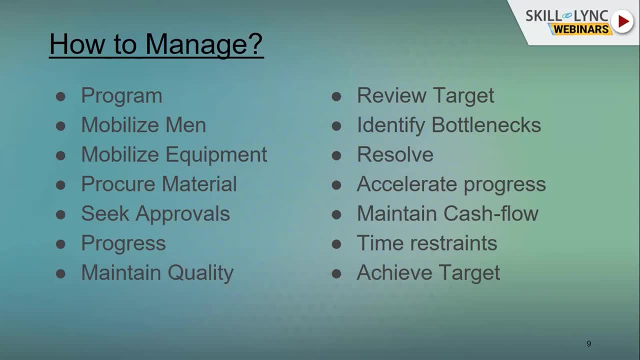 project and how we will go are going to tackle that, Say example, sometimes you know labor is also not available at the site, so do we penalize the contractor for that? no, we should be, you know, raising our hand to him, that you know definitely we will recover this after couple of months. let the 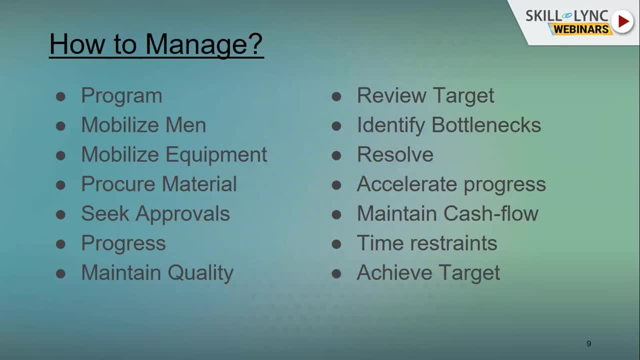 things get sorted out. it's not about, you know, you are so emotional to that contractor and you are giving something. it's just about being a corporate, being a being, a, you know know, being a good human being also. sometimes you have to manage all those particular things and 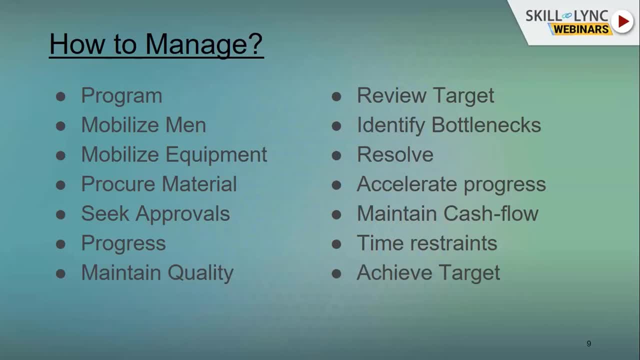 maintain. so now actually the major crunch here. this example is a cash flow. so if cash flow management won't be there, definitely executor or engineer will not perform to its efficiency, so that cash flow management, he has to manage the cash which is coming from the sales of the 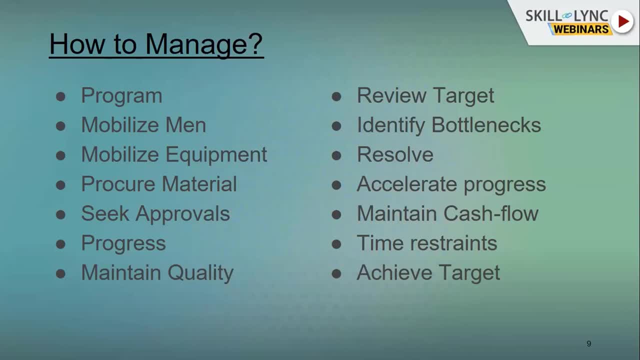 purchase of the flat or something from the owner. it should be planned in that way that no one will be affected, nor owner will be affected due to the work, nor contractor will be affected, so that you know they will maintain the smooth flow of the work throughout the project and achieve the target as 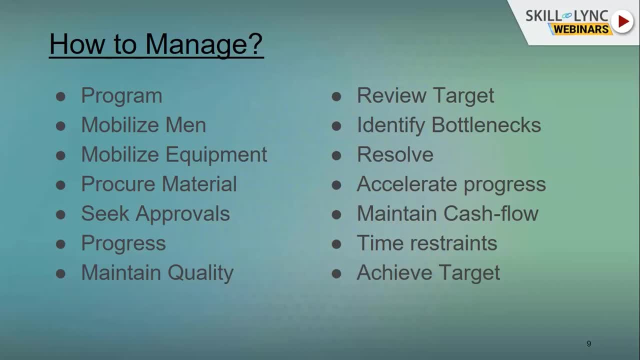 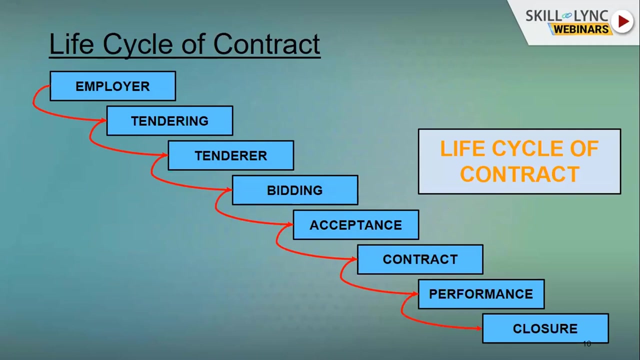 per the desired timeline set by them. so i hope you are clear with this particular complete process of, you know, contract. actually i mentioned in a vast ways, so now, life cycle of a contract. it will, as i mentioned, that it is starting with the employer. employer gives the tendering, so now tendering is nothing. 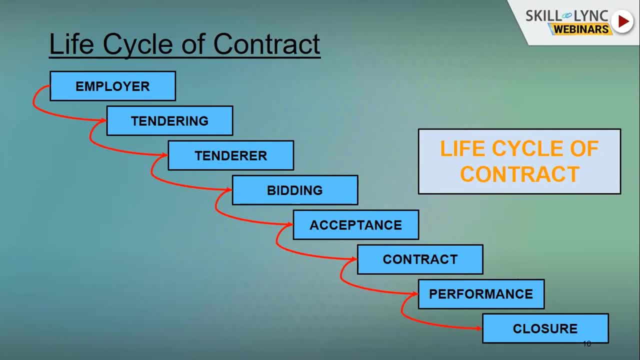 but tendering is nothing but the data where everything is compiled: your BOQ, bill of quantities, your drawings, your conditions of contract, different types of data, your payment terms. everything should be there in one thing. that is nothing but a tendering. it called as a tender. we. 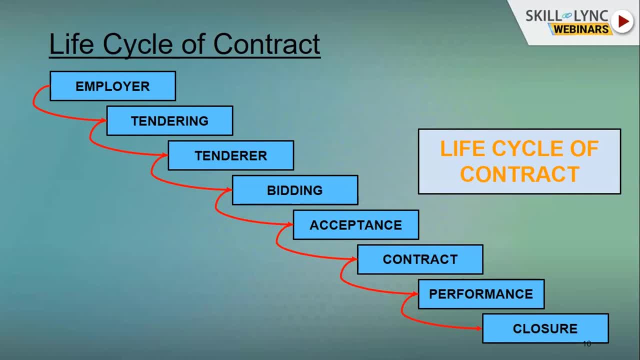 normally use that particular word in our professional language, but that process is called as a tendering, followed by tendering the tenderer. that tenderer is nothing but a person who is going to fill that tender for the employer. so there are n number of tender depend upon the qualification criteria set by the employer. 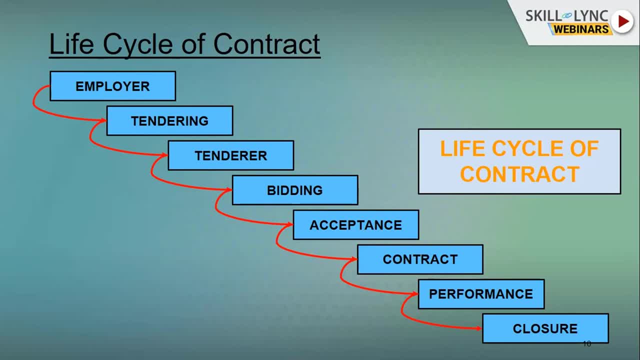 he will going tender, will going to code to the employer. followed after tender. there is a process called as a bidding. bidding is nothing but you know, sometimes there is a e-bidding directly: l1 contractor awarded their work, but sometimes there are corporate companies they allow for the official. 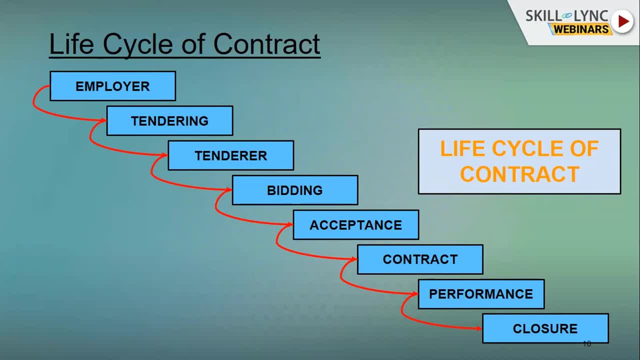 bidding or a virtual bidding, in which they will say that we have this much budget or we have this much timeline you are trying to convince the contractor will complete this work within this timeline, within this budget. so we will going to award that work to the certain parties. 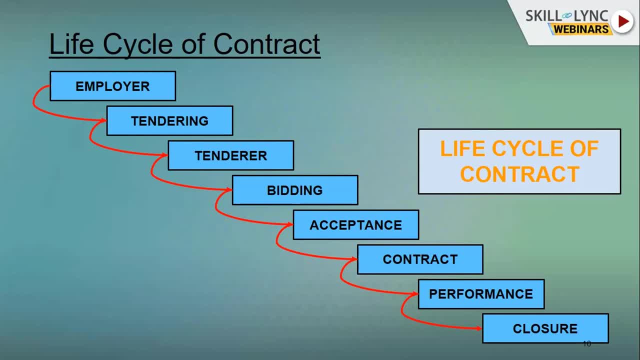 then the major step is nothing but the acceptance. acceptance of a contract by an executor is a major point. where contractor or executor is accepted, every detail, every detail aspect of tendering, including technical, including commercial, and he is now bound to do the job as per the tender to for the employer till completion and that acceptance. 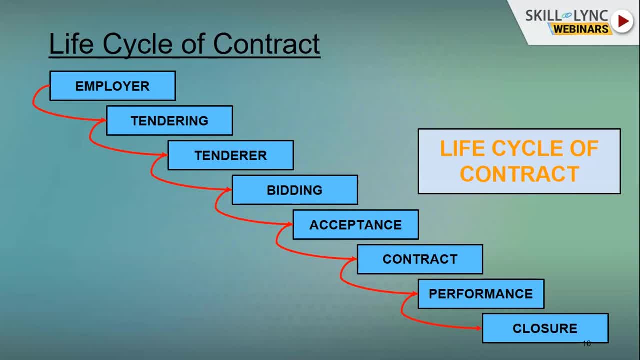 should be signed by the authorized person from the executor so that in case of tomorrow any dispute will come, there shall not be any issue tomorrow. so this is a you know very good note. tom dick and harry of a company can sign the acceptance of contract unless it is authorized. 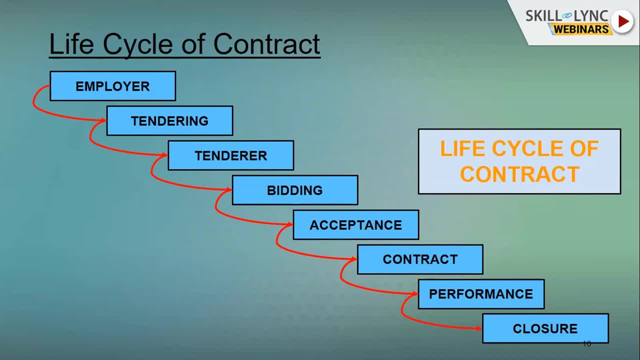 then definitely otherwise authorized person for the organization only can sign this acceptance of contract copy followed by the performance and the closure. as i have mentioned, that performance and closure is a very big topic, and closure is also a big topic because sometimes do happen that projects end up with the dispute or some micro detailing or delay, etc, etc. so how you will going, 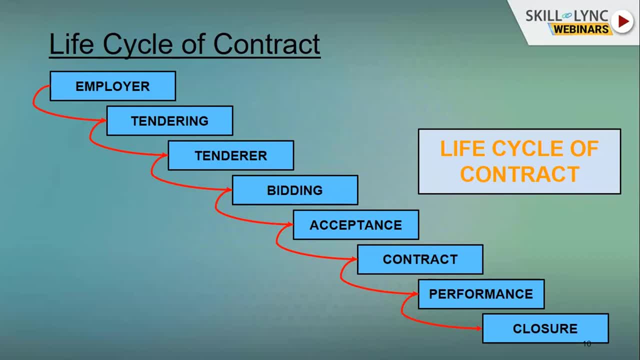 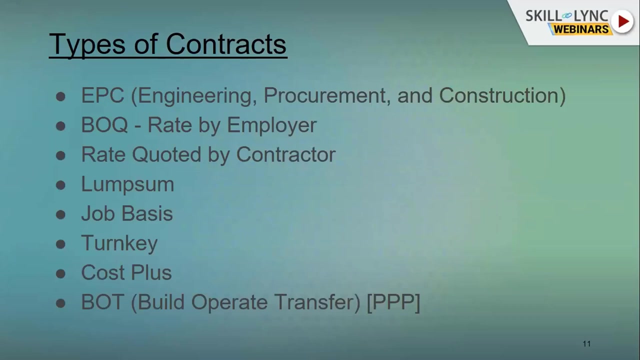 to handle that and how you will come out from the project. being a contract manager, a target is to start and end the project as per the employer's requirement, because any delay or anything would be trouble for the organization and itself for the contract manager. so to proceed further, so i have mentioned the five to six types of contract we 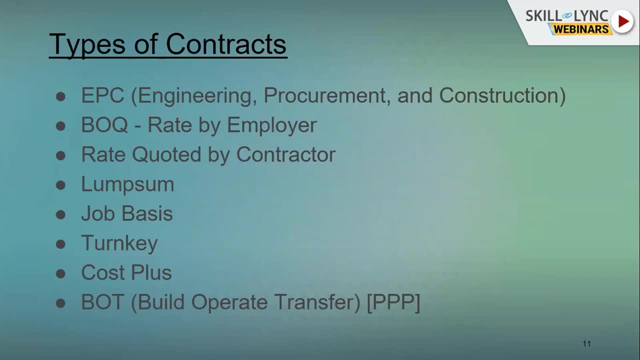 used to deal with in our construction industry. so one day a employer comes, and you know, a employer or a ceo of the company, say example, i would like to establish my twenty thousand square feet commercial office and i- i don't know anything about what is the. 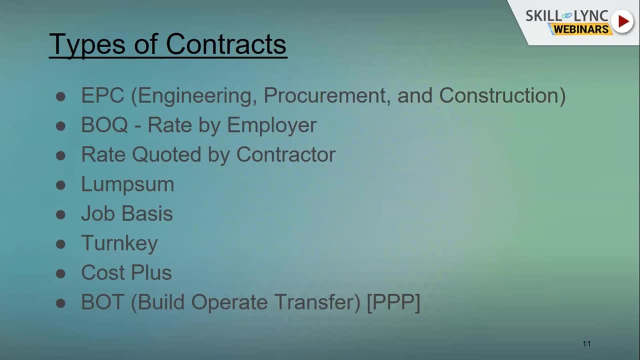 engineering aspect of office. i will just give you a number of seats required for my employee. i will give you the mds cabin. number of cabins required, number of toilets requirement. and everything can be done by a contractor, say example, starting with the engineering aspect, procurement and construction, then that contract will be nothing but a epc owner will say only that i need this. 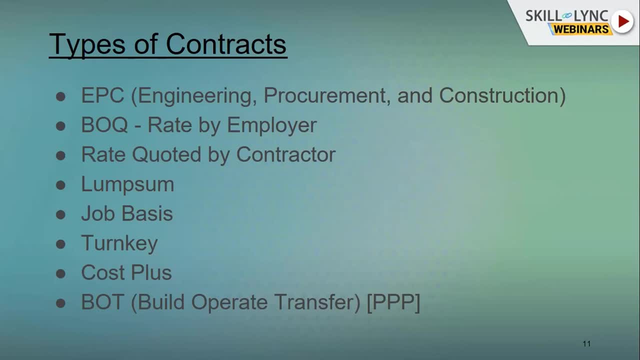 particular office. under this style, under this requirement, within this budget and within this timeline, every engineering aspect can be designed by the contractor. here then boq, rate by employer. boq is nothing but bill of quantity rate by employer. so here what happens? that you know detail, boq has been given and the rate quoted by employer owner himself code, the unit rate for. 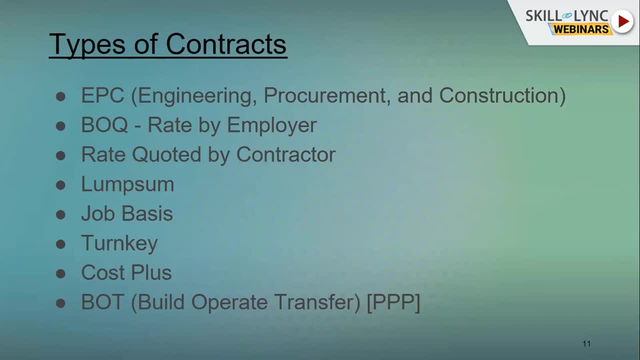 that particular item and arrives at a certain total of the project. so contractor has to agree to re to walk at the same rate so that you know they will going to have the context. so such a contract will be called as a boq rate by employer. the third types will be rate quoted by contractor. in this a 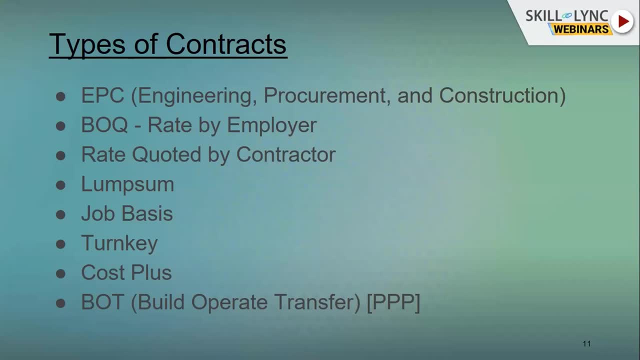 contract will be called as a boq rate by employer so that you know that the contractor has to quote the rate with respect to the boq and its unit rate. whatever detailed description has been mentioned in the boq, that contractor is agreed to mention and use the same make of the material and. 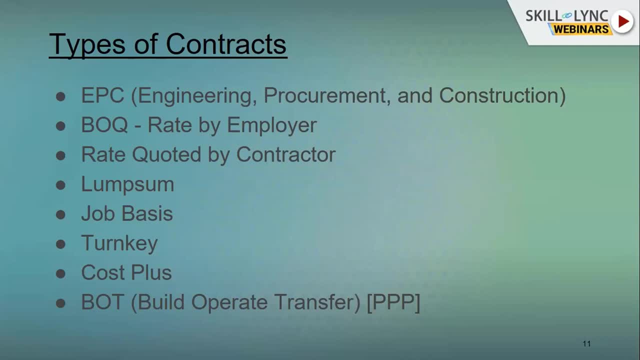 accordingly. he will going to quote it. fourth one is a lump sum basis. lump sum basis contracts are, you know, majorly, uh happens same, is kind of a epc but not engineering procurement kind of a thing. just a requirement has been given to the contractor and contractor will work on the 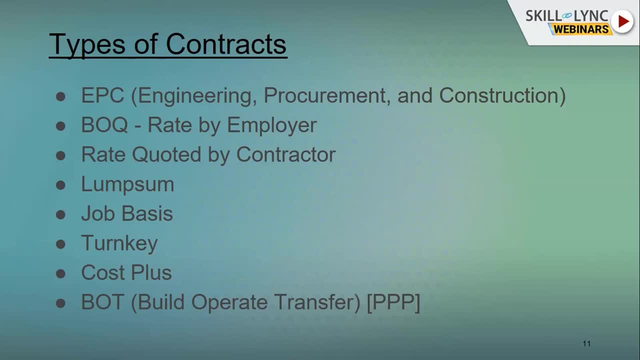 lump sum amount only pertaining to that requirement this contract may lead to, uh, having the biggest disadvantage is that when employer wants certain certain change in the layout or something like that, so that that is very costly in terms of lump sum, because your rates have been finalized as per your earlier requirement, any changes contractor will charge you. 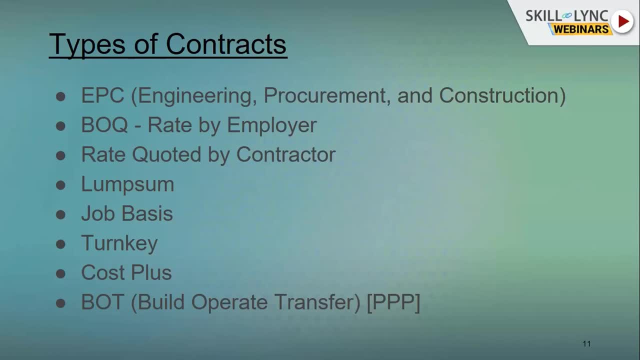 more, considering that the same part will be executed by him only. so such a work, you know it's. it's depend upon how, and then what kind of project uh required for such a work. otherwise, it is better to not to go with lump sum contracts. next is the job basis. job basis is nothing but as per the job. 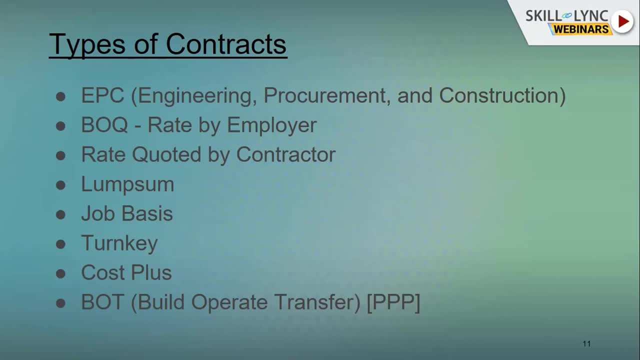 just contractor has to code and has to perform the job. so now, turnkey, turnkey contracts is nothing but design and build. i'm repeating that. what happens? that the complete design of a layout of an office, to its execution, everything done by a turnkey contractor, we can say that turnkey. 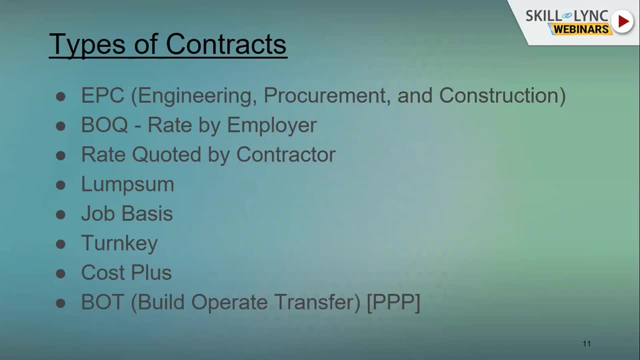 contractor. uh, epc is a part of turnkey contractor but turnkey contractor cannot be part of epc contract because in turnkey we are not going to evaluating the engineering part, we are only doing the design of the contract. so we are not going to evaluate the engineering part, we are only doing the 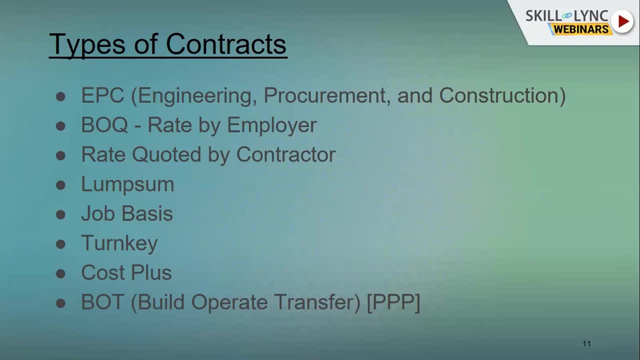 design and build and in epc we are doing the engineering, procurement and construction. so cost plus, cost plus contract is the thing, but where, as per the currently, as per the terms and the condition or the drawings contractor has to carry out the work, he has to submit the bills of a 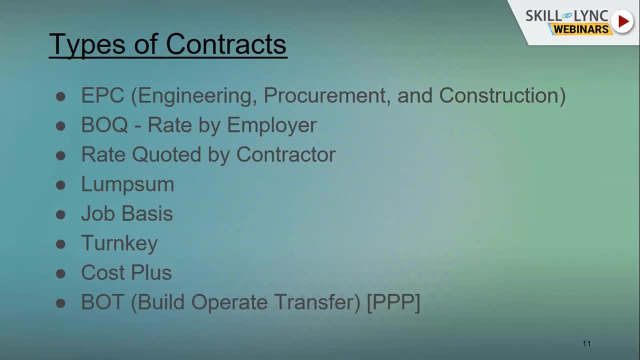 supply of material as well as the labor charges, and employer and executor will agree to add certain profit margin in on that particular cost it that contract will be called as a cost plus contracts. so cost plus contracts are generally in the terms of a small contracts value, where you know. 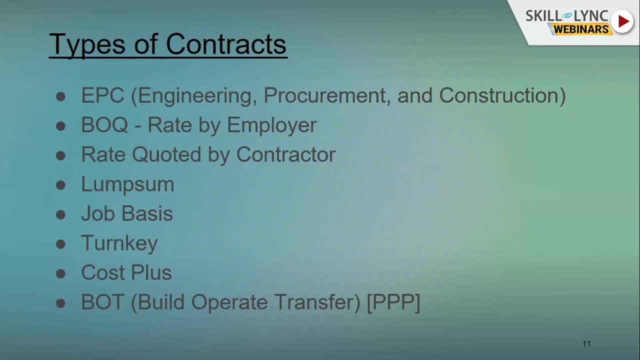 where the small amount value- you can say a small contracts- can be work under this particular cost plus contracts terminology. uh, the next is a bot built, operate and transport. this is a major contract where, you know, majorly, we will find this contract in government sector, where 70 to 90 percent of 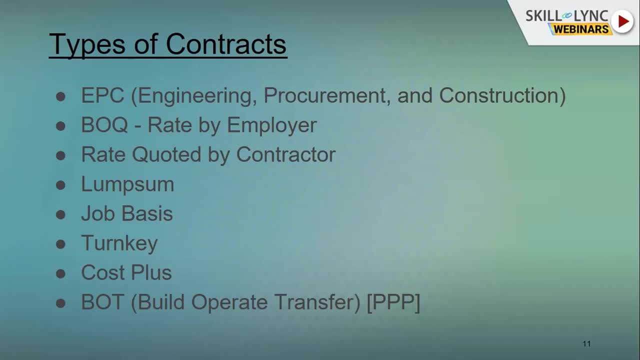 government. big projects are running under this contract. i will give you one example of here that a mumbai metro is running by mmrd but currently build, operate and transport by reliance. so reliance will- uh, reliance will operate for a certain period, say around 20 to 30 years. 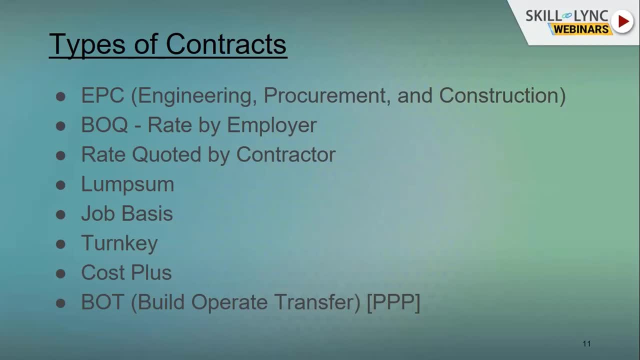 depend on the target customers or depend upon the target travelers and their unit rate, so that period is designed by an third party or example reliance in such a way that they will going to earn some profit margin after they break even point. so this is a joint call between government. 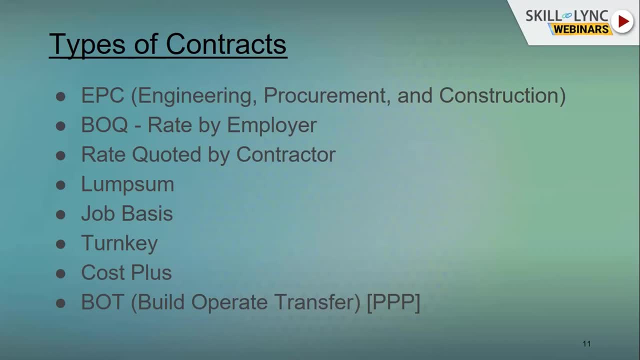 and reliance- mmrd and reliance- in such a way that they will going to survive or they will going to maintain that property for 20 to 30 years- depend on the agreement- and after 30 years that complete property goes to the government as a government entity in this. why. why government goes to this? 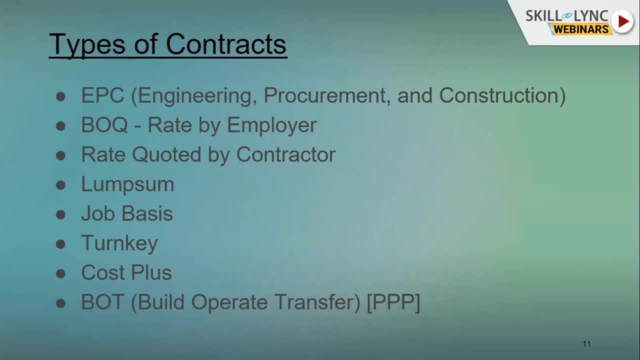 beauty. because of the budget constraint and the employment example, the bigger companies will take it up the part of the government load financially and it is a win-to-win situation for both the party. considering the future development of the India example, Bandra Worley ceiling, MMRDA owns that particular project and MEP. 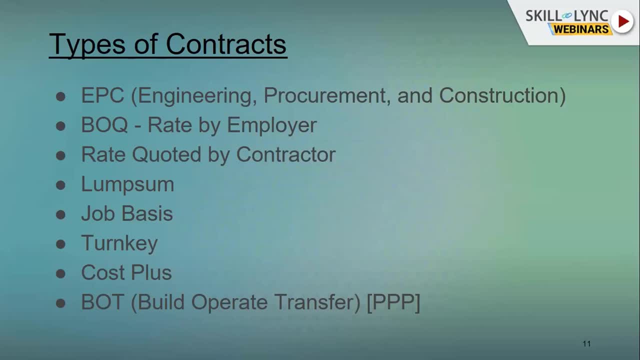 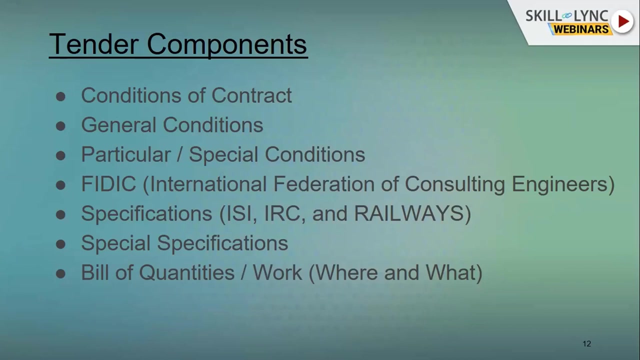 contractor is going to MEP as a contract with MMRDA for maintenance and collecting the toll on behalf of government for 20 years. so, as I have mentioned, there are different types of contract. so you know, as I have earlier mentioned, that I will just going to focus. 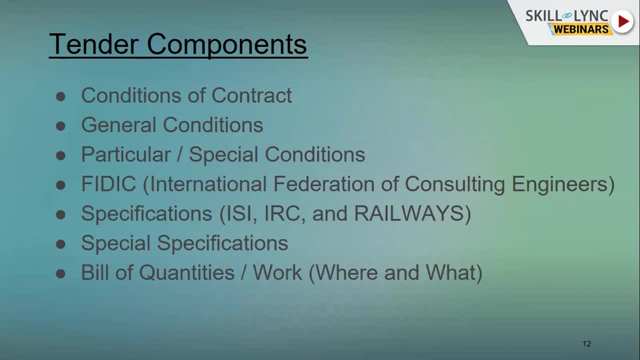 one aspect today that is nothing but a tender. so this is the first point where a contract manager has to act upon it. after you know, once we receive the confirmation from the board of directors or the management, that we have to start this project. so this is the 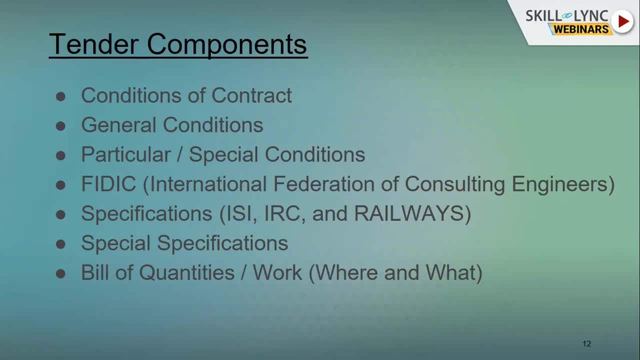 first thing that contract manager has to start. so what are the things that you know? tender, tender should have to avoid the contract. Avoid ambiguity in the future stage. first, there are three types of conditions: conditions of contract, general conditions and special conditions. so first we will start with the 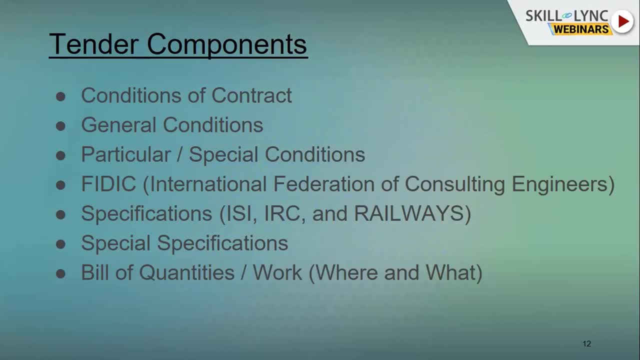 conditions of contract. conditions of contract in which you know everything is mentioned regarding material rate, labor rate, what is the timeline for that particular project, how the project will going to work, what are the penalties, what is the mode of payment. I can't cover that. so you know, all these things are there and then we will go into this chapter. 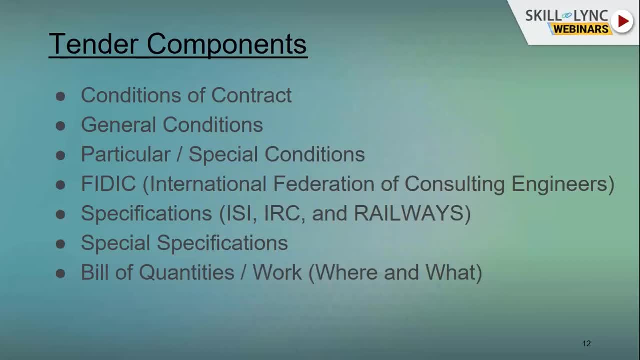 of terms and conditions I have mentioned, and the last that they have mentioned is the amount of security deposit. security deposit is nothing but, you know, amount mentioned which has to be paid by the contractor after allocation of the work, just to ensure that they will going to work as per our terms. 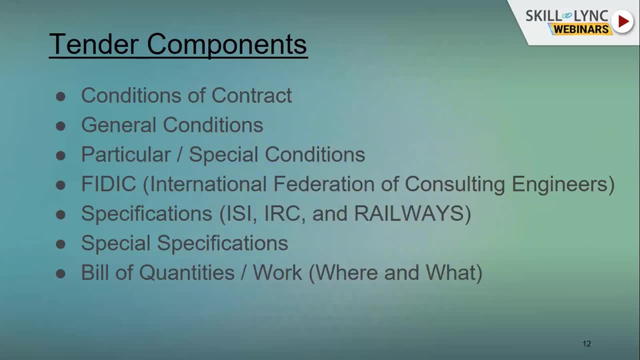 This is nothing but a security. after this, It's a security scheme. So it's a security scheme be given to the employer after allocation of the work. example: general conditions. general conditions are nothing, but you know who is going, who is employer, who is engineer, who is executor, so just. 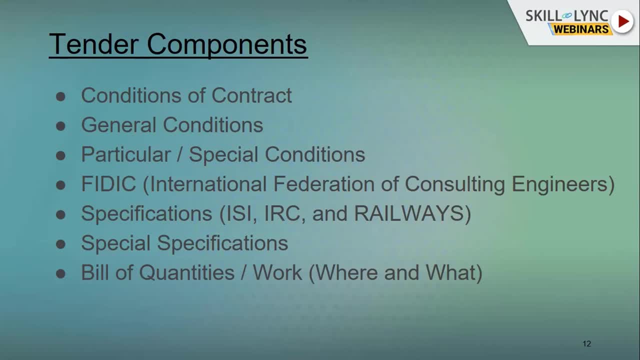 definition of entire. all the stakeholders and the concerned people in the contract they are mentioning here- and there are sometimes general conditions- may have the procedure for claims also, that how someone will claim extra or someone will claim other things, what they are not able to claim into the contract, say. the third point is a special condition or a special contra special. 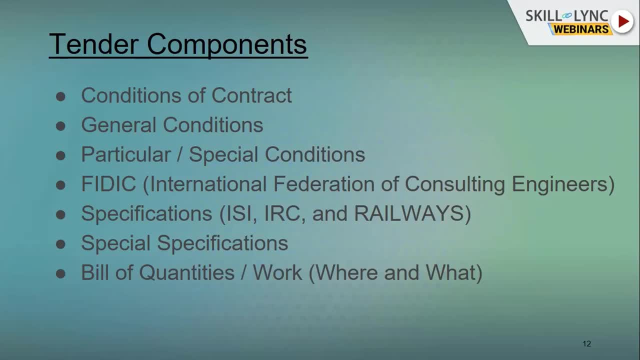 particular conditions. so in this this is nothing. but in addition to the condition of the contract there are terms and condition that sets out the rights and obligations of the party. this is nothing but to have the rights about their both the parties. this is not mandatory in all the contracts, but definitely. 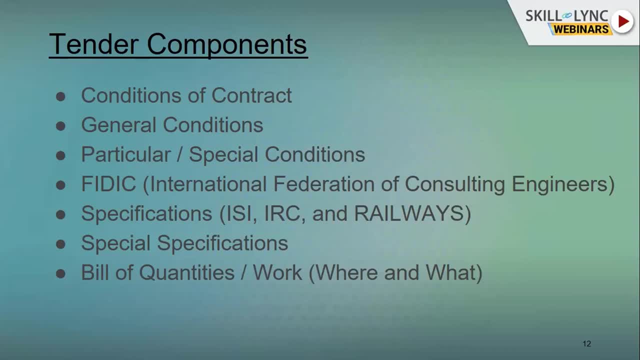 we can mention depend on the types and the works of the contract: fidic. fidic is nothing but international federation of consulting engineers. they are providing a on. fidic is an organization which provides a contract agreements and they are continuously they are continuously monitoring the progress of the works of a different, bigger projects and they are continuously modifying. 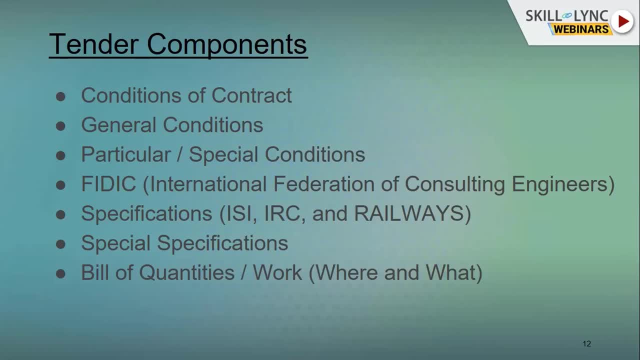 the contract conditions from fidic we can identify, depend on the task of the project. we will take out the conditions and we can fit in our project. what are the suitable for our projects? next is the thing, but the specification, specification is. you know that, say, example. if i would like to, 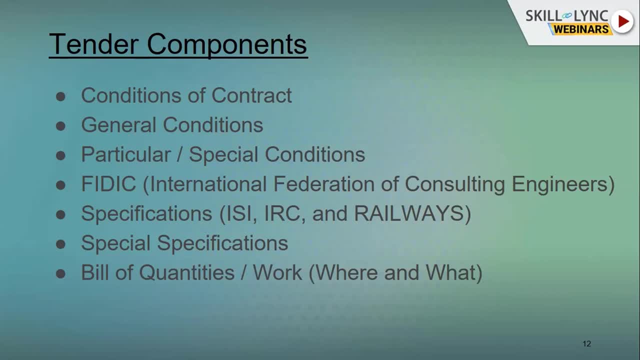 i would like to start with my foundation specification. so what kind of excavation i need, what is the quantity, how we will going to excavate it? then specification for RCC. what is the grade of the concrete that i will going to use? what is the grade of the? 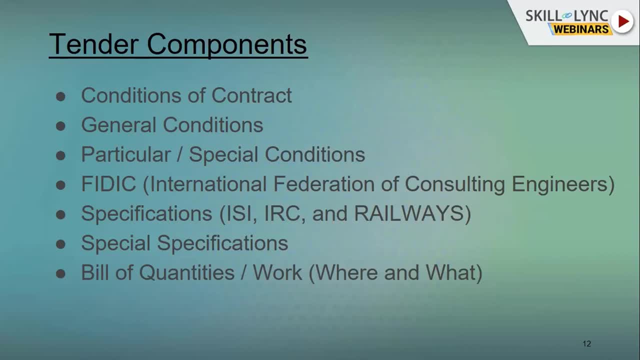 steel. i will going to use, as per isi example, if i am caring out of project in railways, so railway standards, that all the materials and specification with reference to the standards are mentioned, and to be prepared for one of the part of the tender, special specification, specification, definitely special specification. like, say example, we are constructing one government. 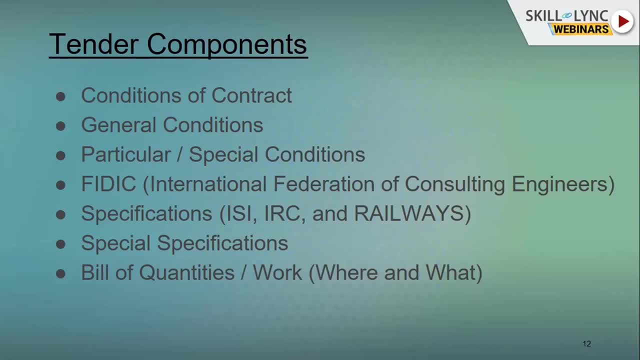 building and they will be requiring a bulletproof glass. so this is nothing but a part of a special specification where a special material need to import by the executor from a different countries and he has to certified it up to their standards and up to our standards and 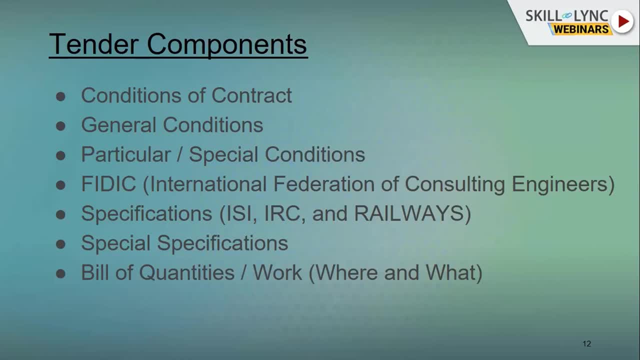 he has to guarantee that you know what are the different needs of the particular specification and that he has to adhere to that. Bill of quantities is the thing, but you know complete detail, item wise specification, along with the unit quantities, and that quantities has to be calculated with the help of AutoCAD.